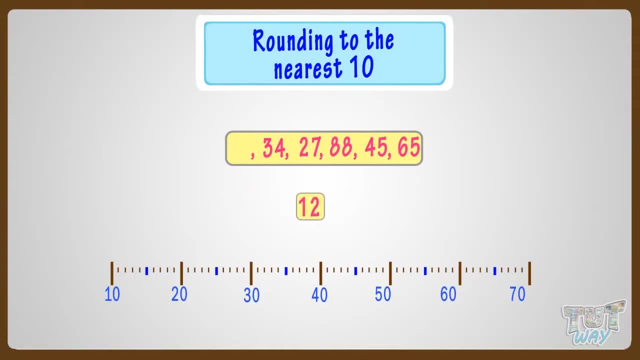 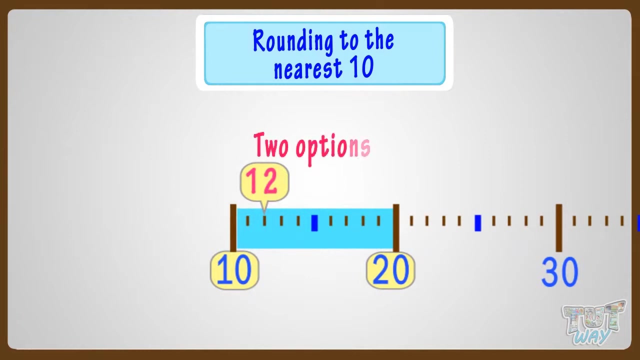 Let's start with twelve. See the number line. Where can you fit 12 on this number line? It is somewhere between 10 and 20.. Whenever you want to round a number, there are always two options. Either we can round it down. 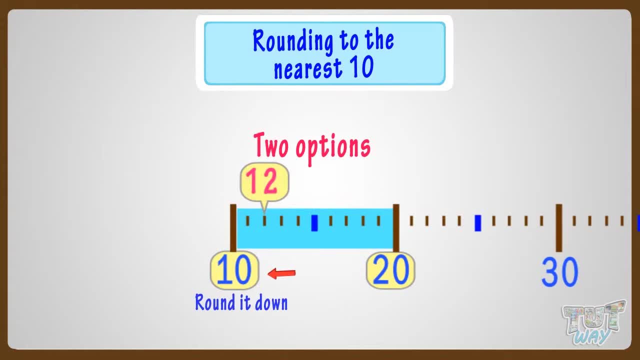 previous 10, that is 10 here. or we can round it up to the next 10, that is 20 here. think which option do you think is more apt? here is a rule to help you. you always have a 5 mark midway between the two tens if the number is below 5 mark. 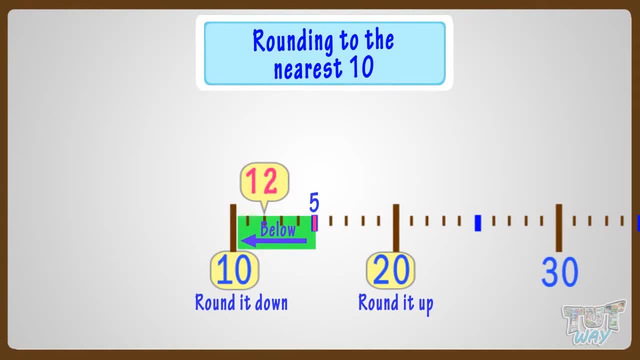 you round it down, that is previous 10, and if the number is at 5 mark or above the 5 mark, you round it up, that is to the next 10. Here, 12 is below the 5 mark, so we will round it down. 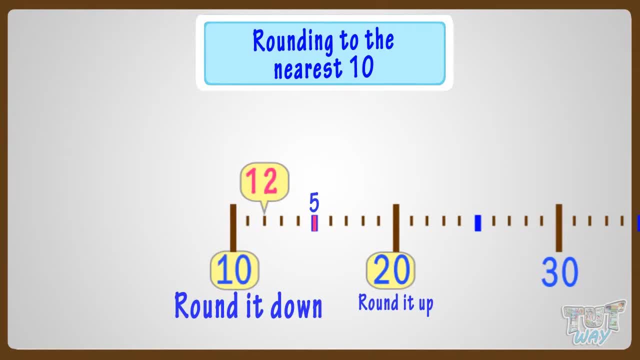 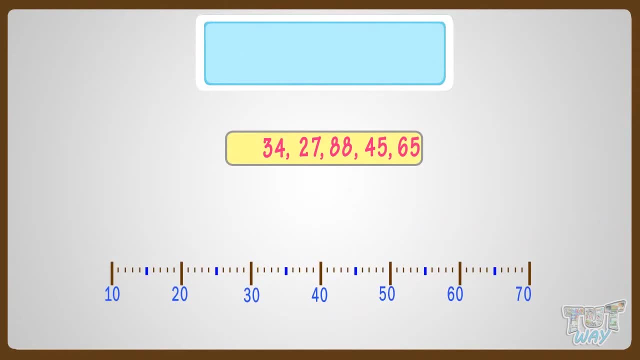 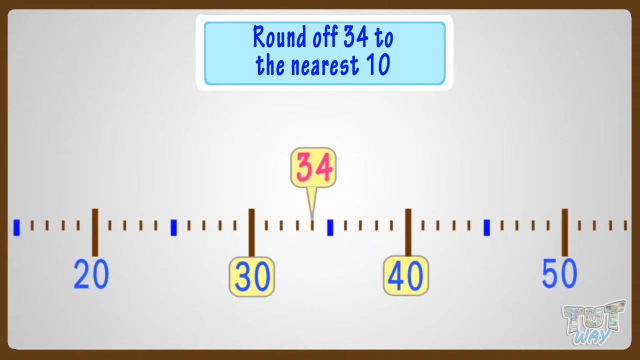 That is to 10.. Okay, now let's take another number. Now we have to round off 34 to the nearest 10.. Where can you fit 34 on this number line? It is somewhere between 30 and 40. And we know, whenever we have to round off a number, we always have two options. 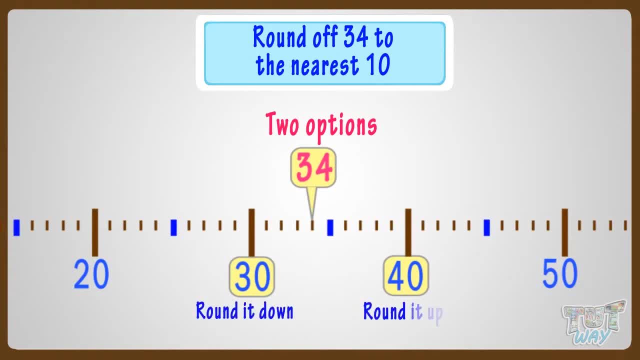 Either we round it down or round it up. Also, we learned that if the number is below the 5 mark, we can round it down, Or else we round it up. Here, 34 is below the 5 mark, so we will round it down to 30.. 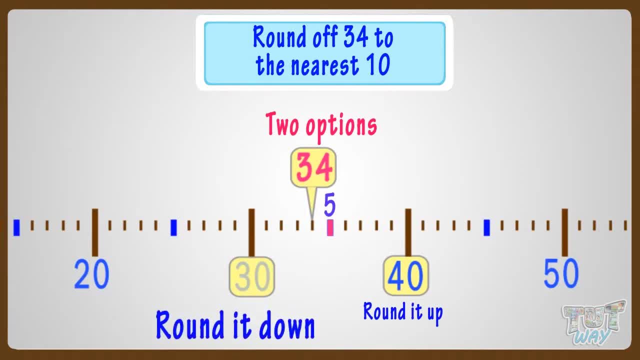 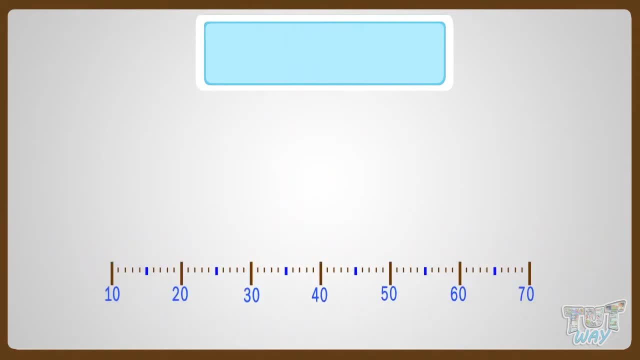 Good, Now let's take another example. Where can you fit 27 on this number line? Here, 34 is below the 5 mark, And we know, whenever we have to round off a number, we always have two options: Either we round it down or round it up. And we know whenever we have to round it down Or else we round it up. Here, 34 is below the 5 mark, so we will round it down to 30.. Good, And we know whenever we have to round off a number, we always have two options. Either we round it down or round it up, And we know whenever we have to round off a number, we always have two options: Either we round it down or round it up. Or else we round it down, Or else we round it down. 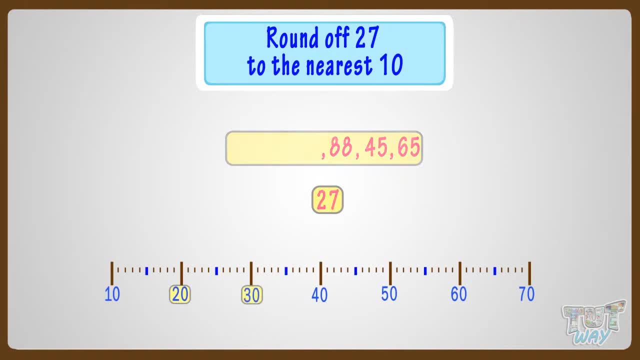 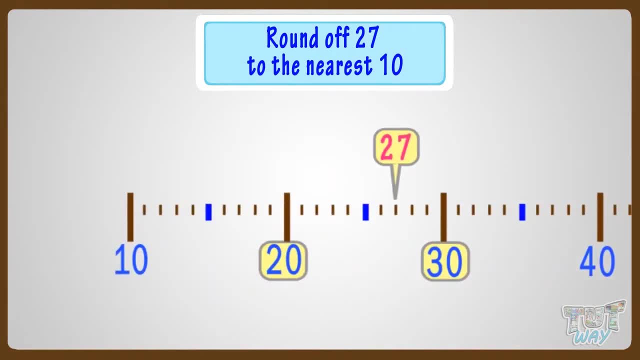 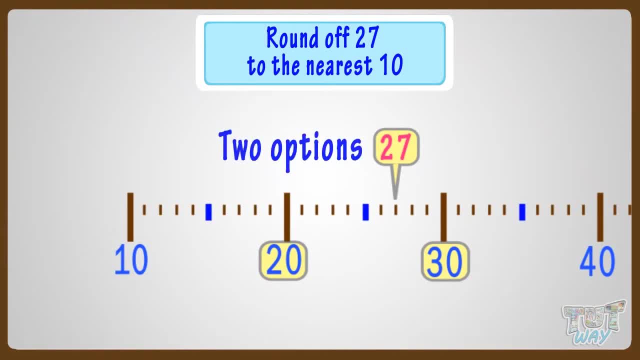 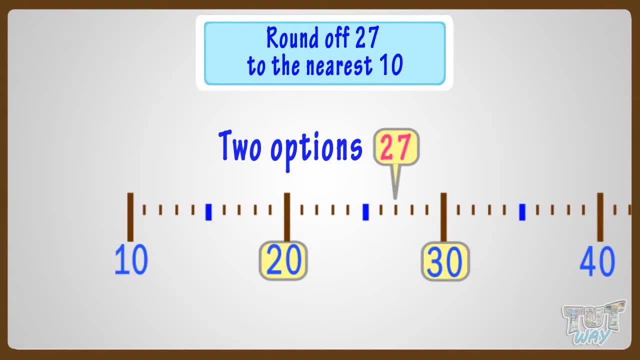 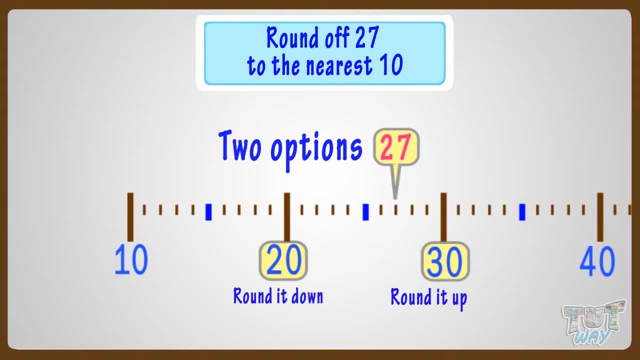